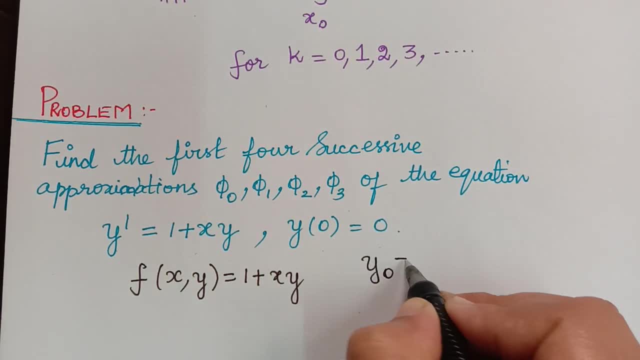 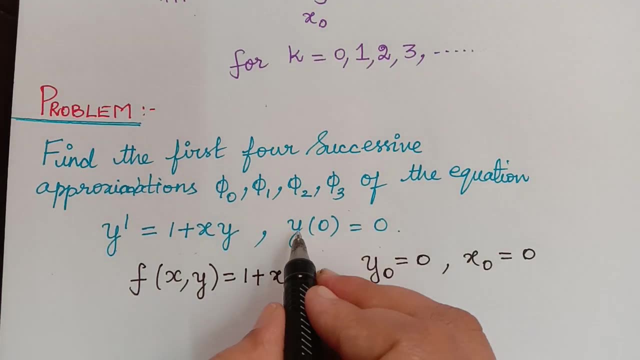 given as 0, which implies that y naught is equal to 0. And what is x naught- x naught is equal- is also equal to 0, because actually this is y of x is equal to 0. That is, y naught is equal to 0. So 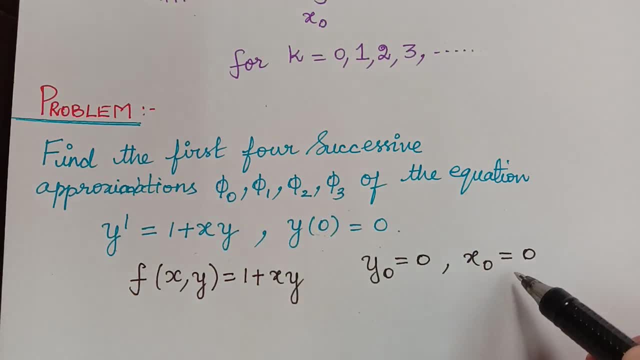 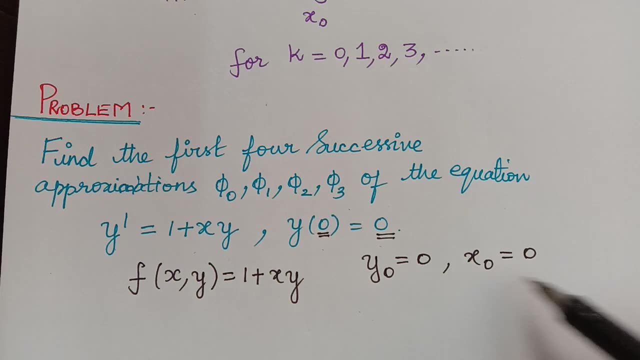 y of x naught. the value of x naught is 0 here. So this gives us the value of x naught and this gives us the value of y naught. So first we have written the initial conditions and the initial value. problem f of x comma y equal to 1 plus x y. Now next, in order to find the successful: 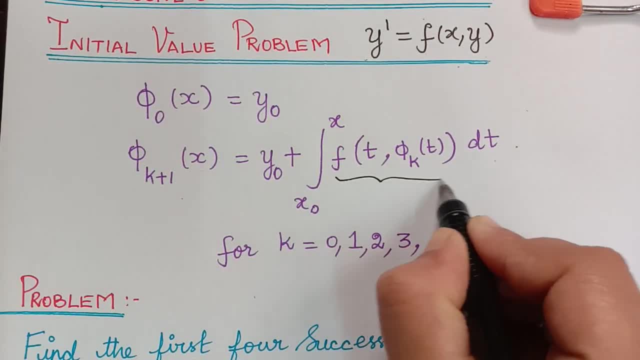 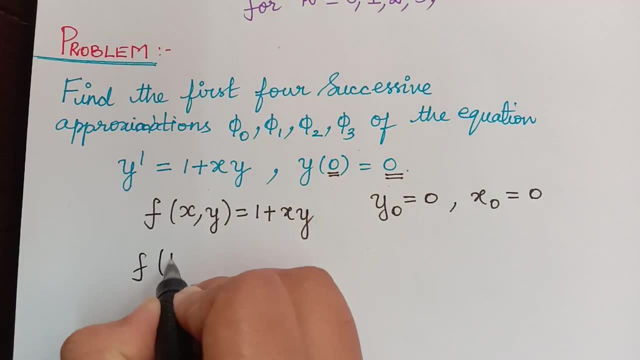 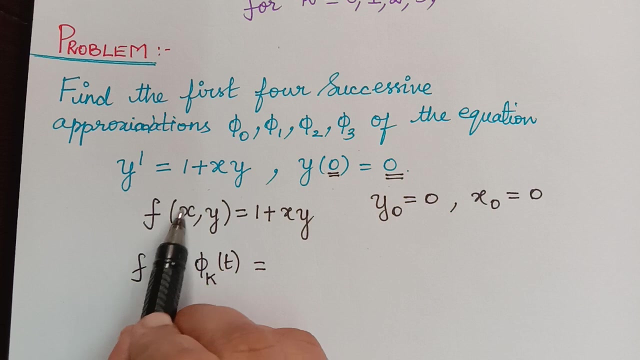 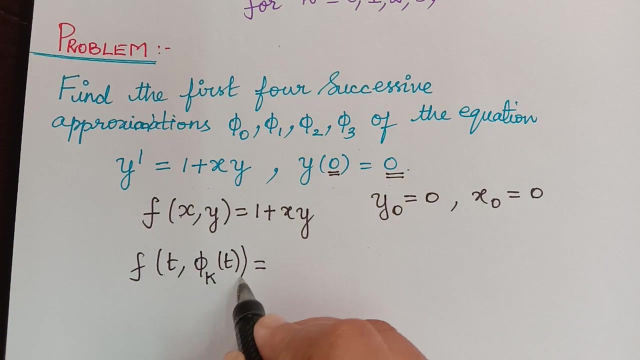 approximations. we shall first evaluate what is f of t comma, phi k of t. So f of t comma phi k of t will be equal to now. in this, wherever we have x, we have to replace it by t, and wherever we have y, we have to replace it by phi k of t. So that will be equal to 1 plus now x is. 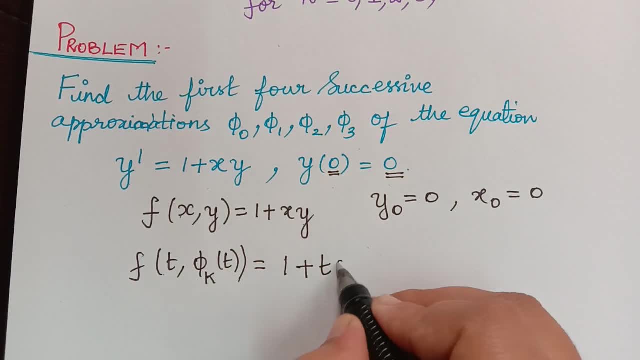 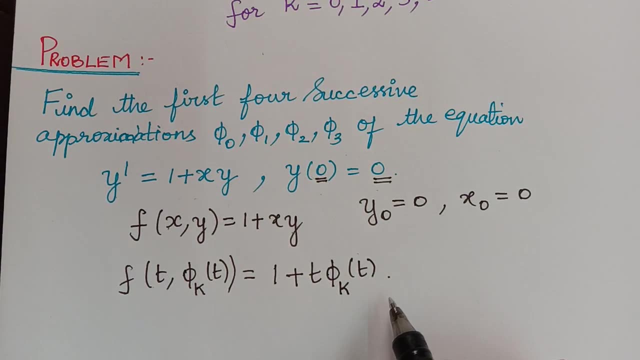 t and in play at the place of y we are having phi k, So we can write phi k of t. Now we shall start finding the successive approximations one by one. So we have f of t comma, phi k of t, and we have 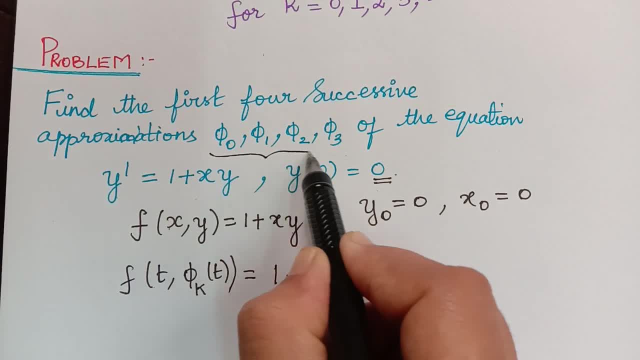 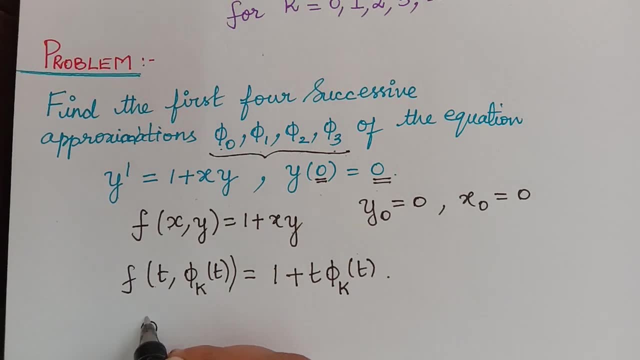 1 by 1.. Now here in the question they are asking us to find the first four approximations: phi naught, phi 1, phi 2, phi 3.. The first one, phi naught, is actually so phi naught of x is equal to y naught. 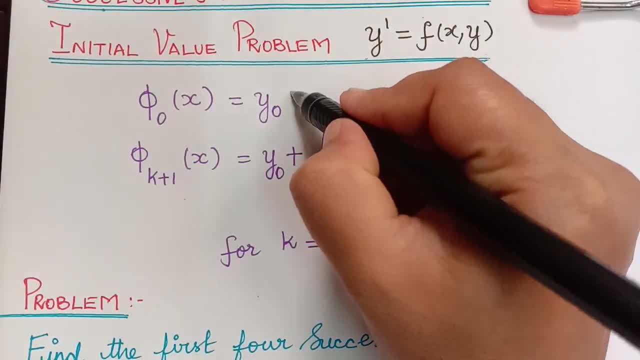 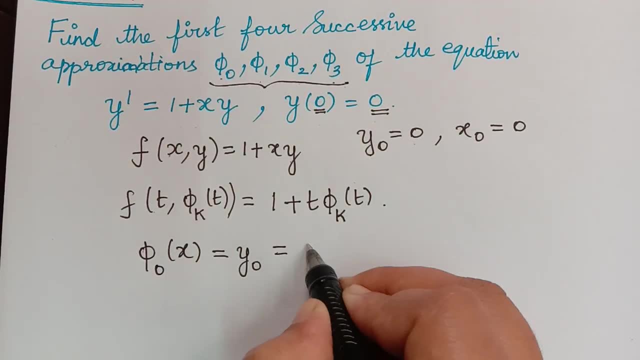 by this. So here we have phi naught of x to be equal to y naught. But what is our y naught here? y naught is 0. Therefore this is equal to 0.. So hence the first approximation, phi naught of x is. 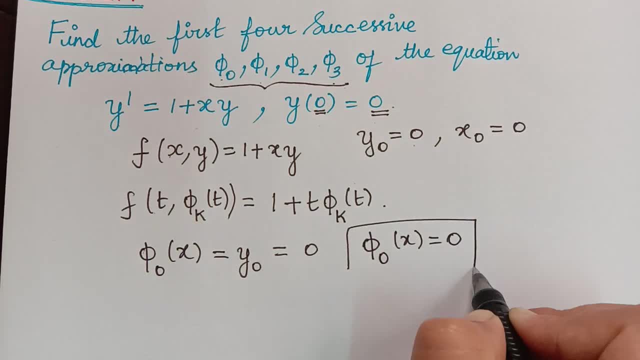 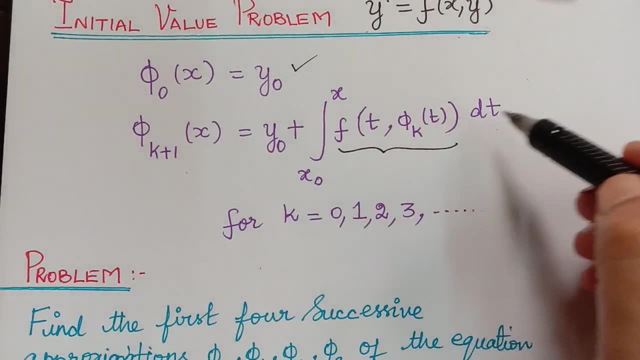 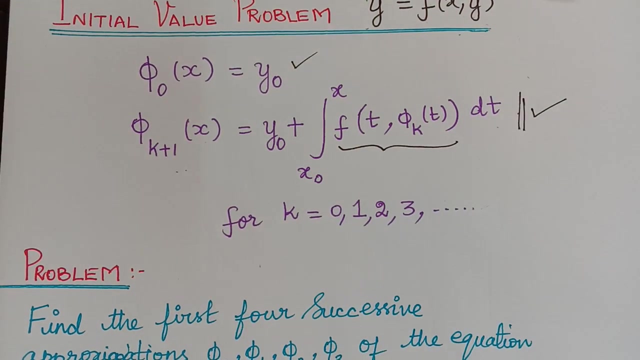 equal to 0.. So now we shall find the second approximation, which is phi 1, for which we need to use this formula. So in this formula we have to put k equal to 0 in order to find phi 1.. So let us mark. 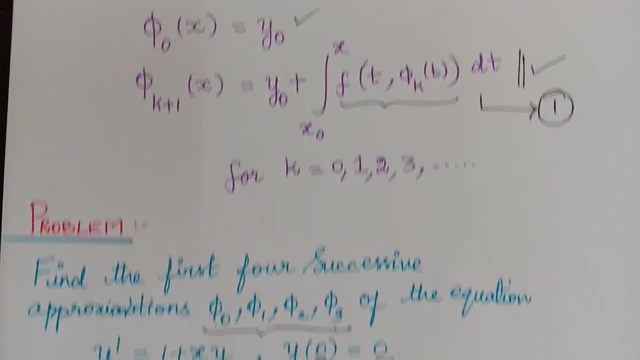 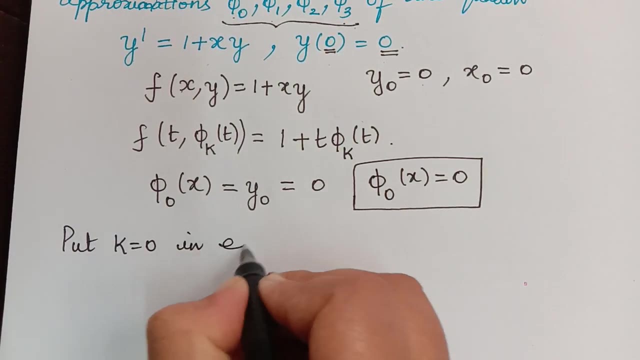 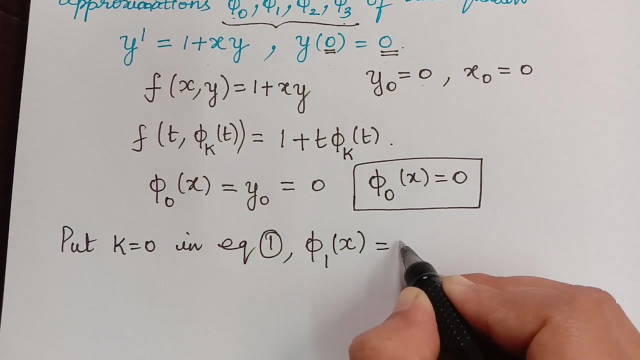 this as equation 1.. Put k equal to 0 in equation 1.. So what do we get? Phi 1 of x is equal to y naught plus integral x naught to x. f of t comma. phi 1 of t dt. 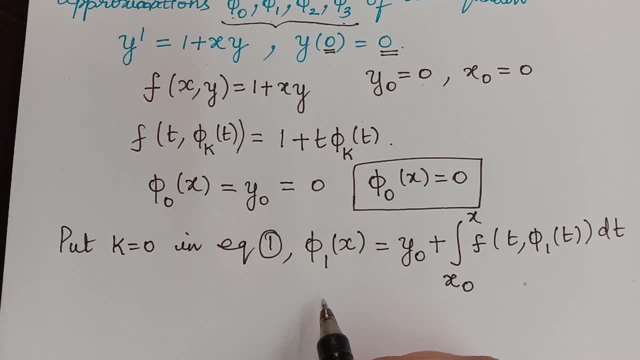 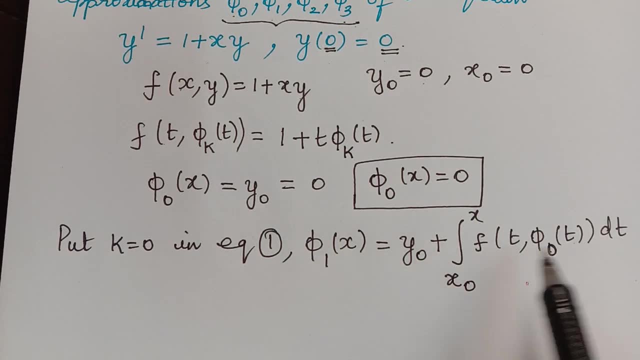 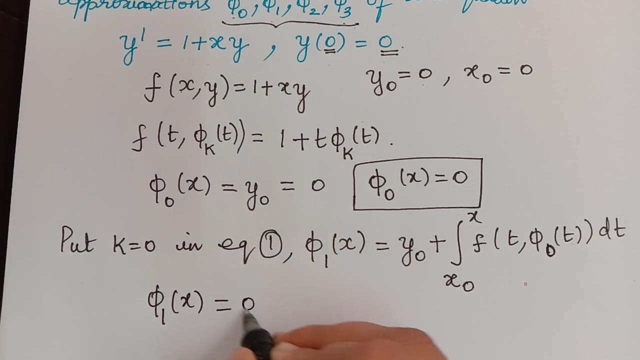 So in general we can also write this as phi k, But actually this is 0 because it is phi k of t and so here is equal to 0, so this will be 0.. So therefore, phi 1 of x will be equal to y. naught is 0 plus. 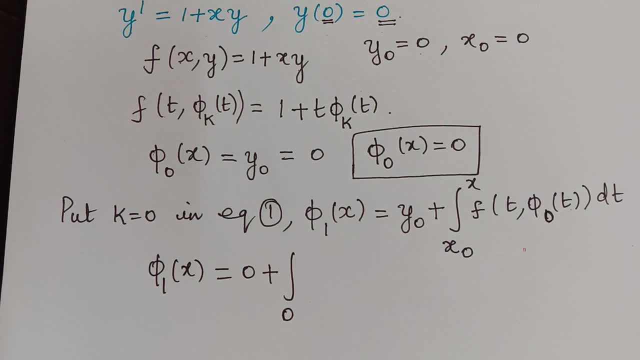 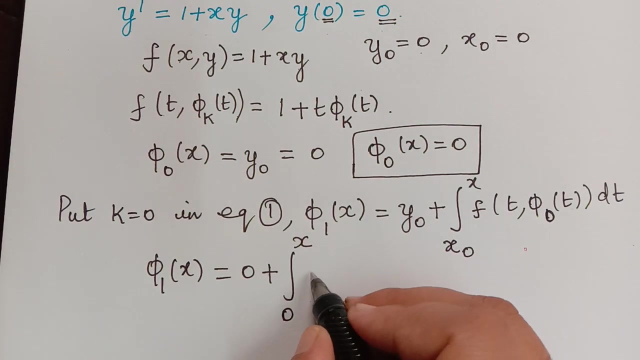 integral: x naught is 0 to x, so 0 to x, and f of t comma phi naught of t, that is f of t comma phi k of t is 1 plus t phi k of t. So now when we substitute that here, we get this to be 1 plus. 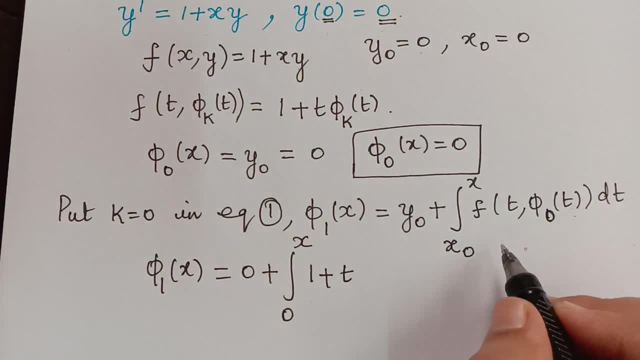 t. what is phi naught of t? it is 0. So 0 dt, and so that will be equal to integral 0 to x and 1, that is t multiplied with 0 is 0. So this term will get vanished. So 1 multiplied with dt. so 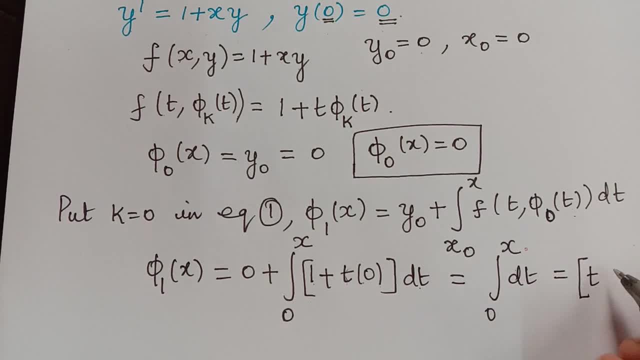 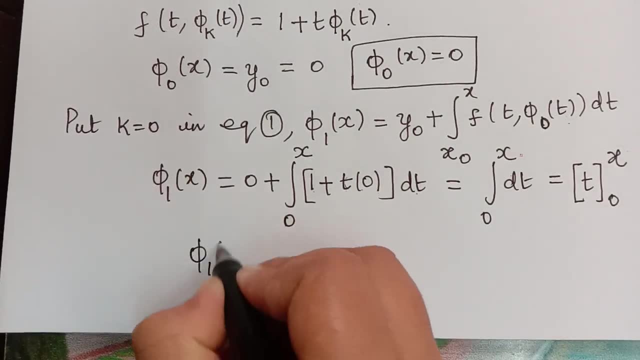 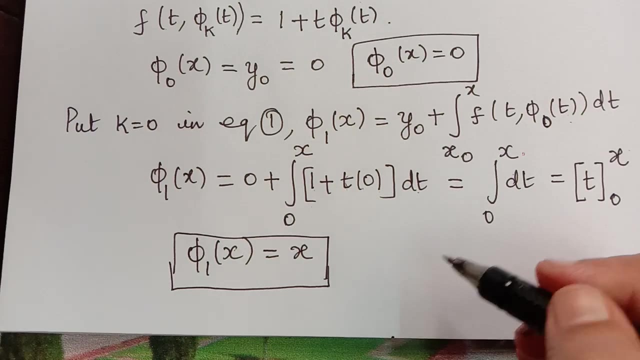 it will be dt and the integration for dt is t, between the limit 0 and x, applying the upper limit minus the lower limit. So this term will get vanished. So 1 multiplied with dt, so it will be dt and the integration for dt we get phi 1 of x to be equal to x. So this is our second approximation, phi 1.. So next we 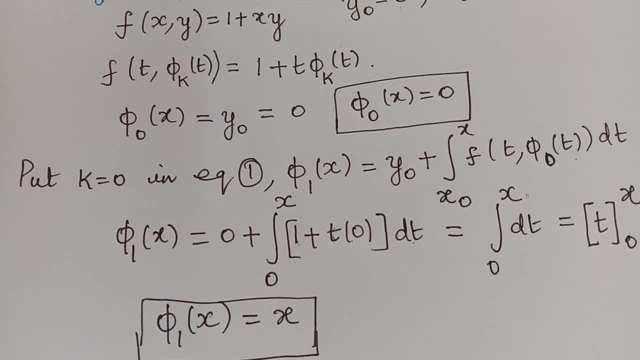 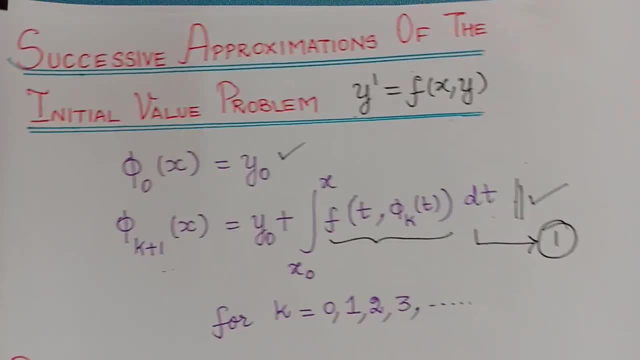 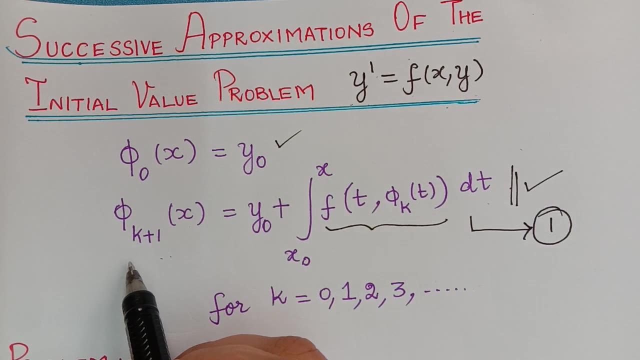 shall find the third approximation, phi 2.. So to find phi 2 we need to put k equal to 1 in equation 1, that is, here we have to put k equal to 1 so that we get phi 2 of x. So let us see that now. 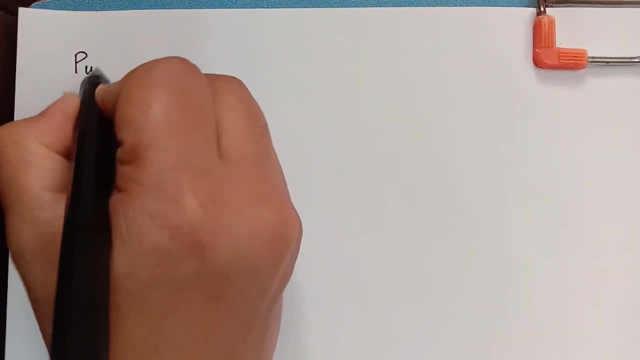 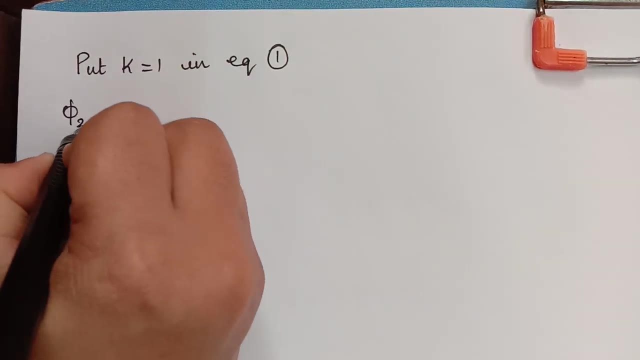 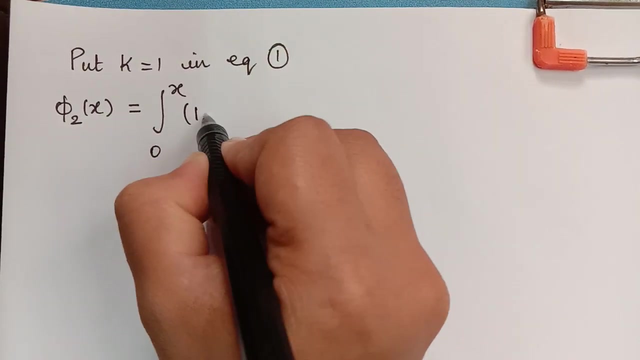 So now we have to put k equal to 1 in equation 1. So that we get phi 2 of x to be equal to integral 0 to x multiplied with 1 plus t, phi 1 of t, dt, and so that will be equal to. 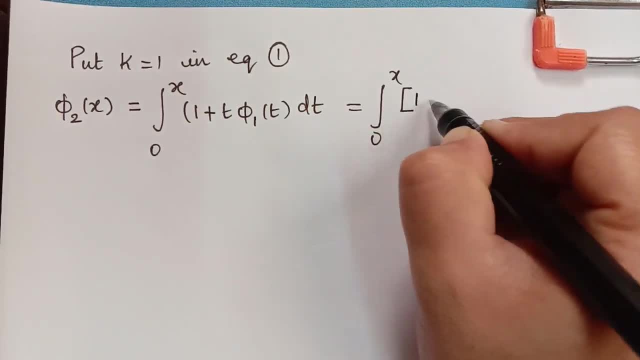 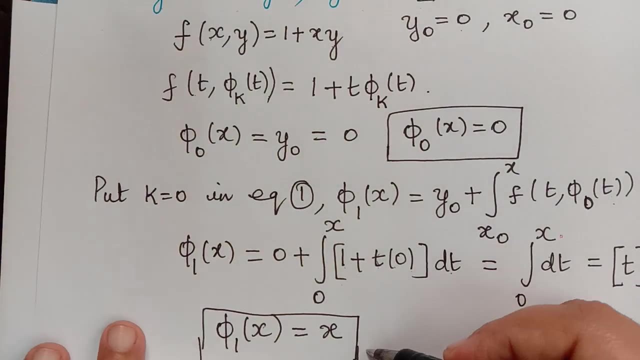 integral 0 to x, 1 plus t. and what is phi 1 of x? So that we get phi 2 of x, 2, and so that will be equal to 1 of t. just now we have got phi 1 of x to be x, so phi 1 of t will be t. so when we substitute that, 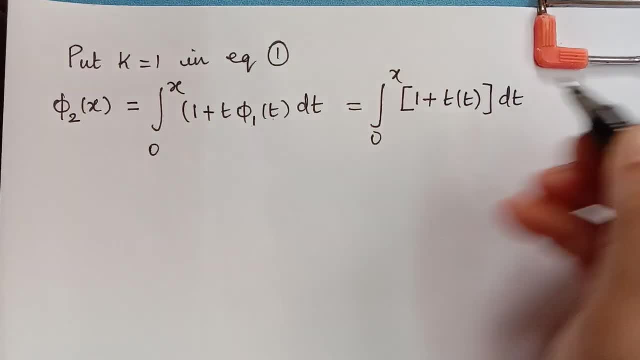 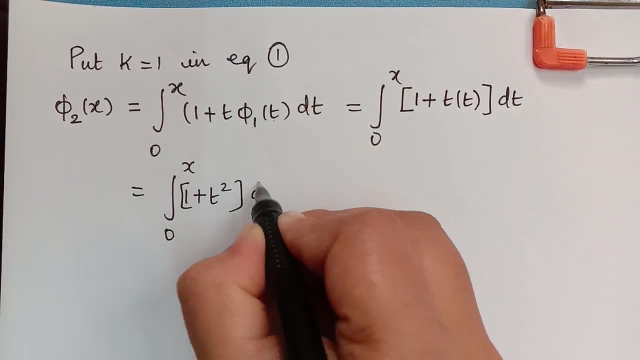 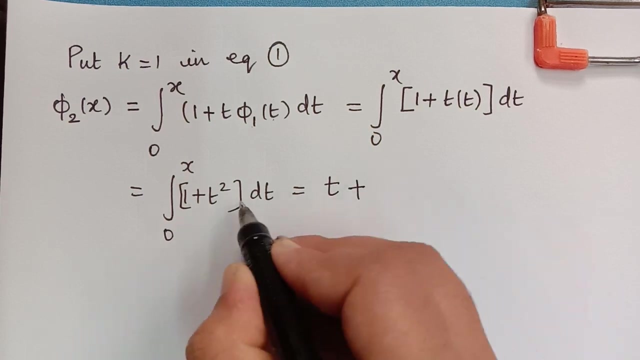 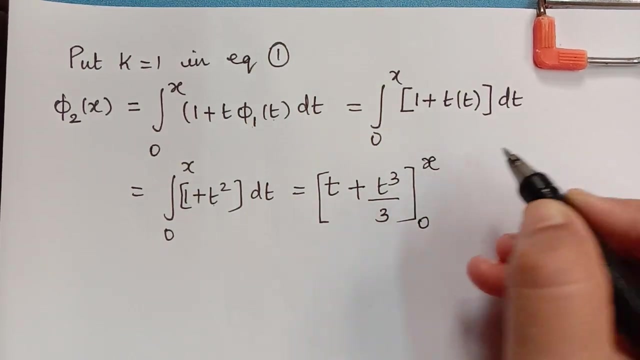 here we have t dt and so that will be equal to integral 0 to x, 1 plus t squared dt. so now, integrating this, we get the integration of 1 is t plus integration of t squared is t cubed by 3 between the limits 0 and x, substituting the upper limit and the lower limit. so upper limit. 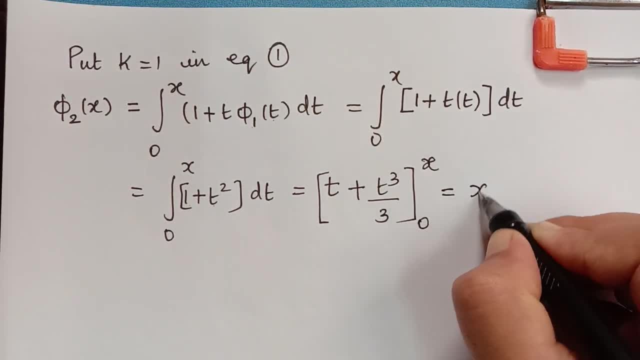 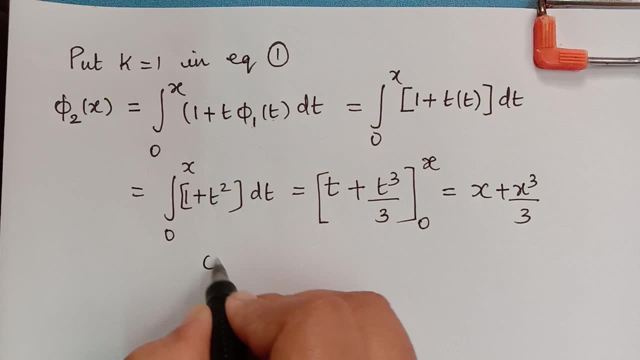 minus the lower limit, we get this to be x plus x cubed by 3, as the lower limit, when substituted, becomes 0. so therefore we get phi 2 of x to be equal to x plus x cubed by 3, and this gives us: 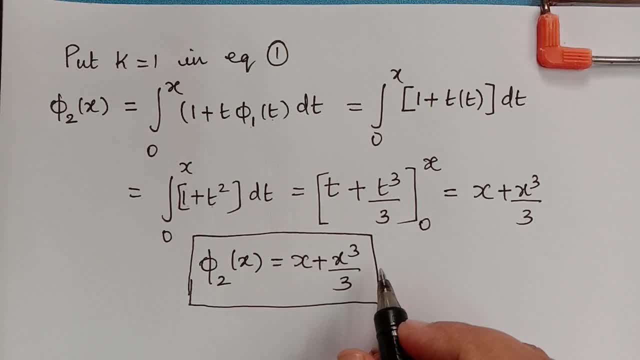 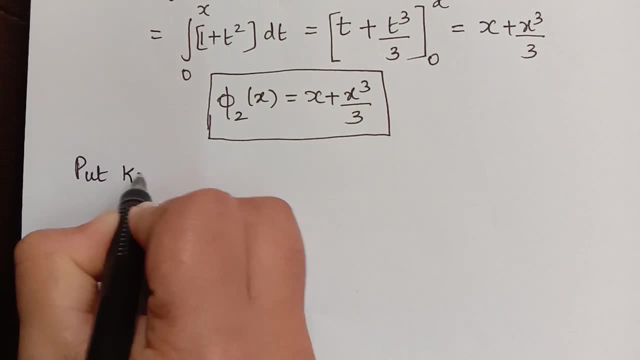 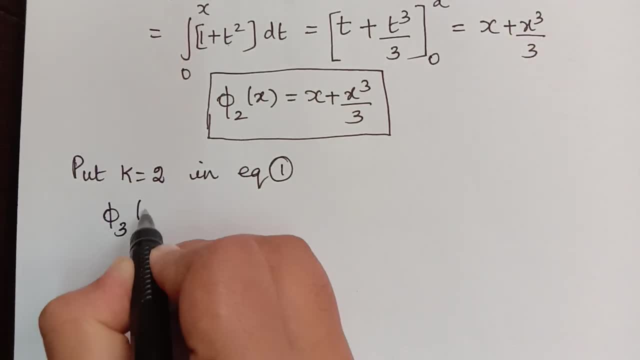 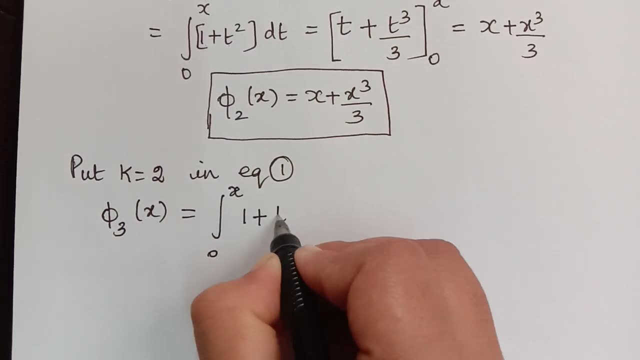 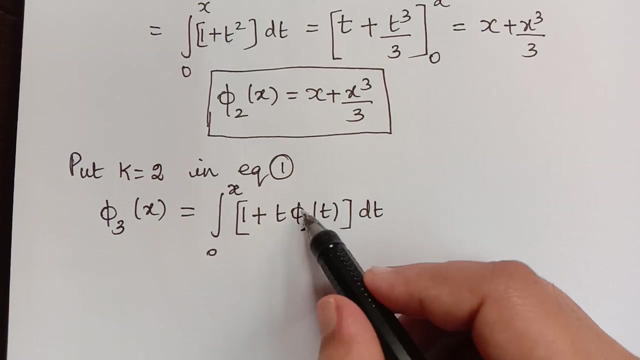 put k equal to 2 in equation 1, we get phi 3 of x to be equal to integral 0 to x and 1 plus t, phi 2 of t, dt. Now substituting phi 2 of t here, that is, phi 2 of t will be t plus t cube by 3, so on. 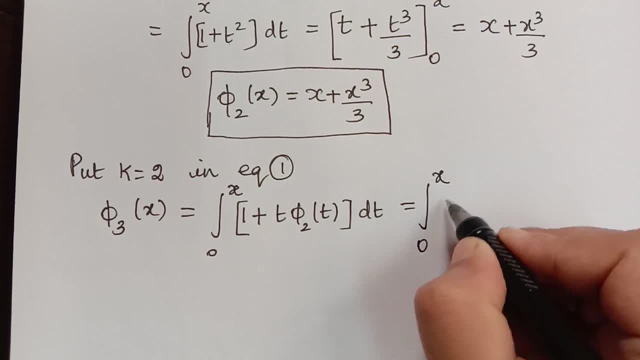 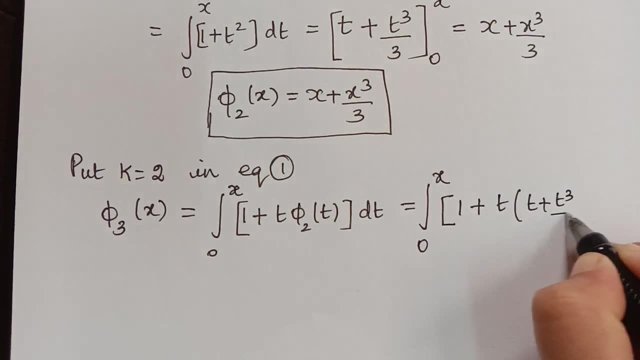 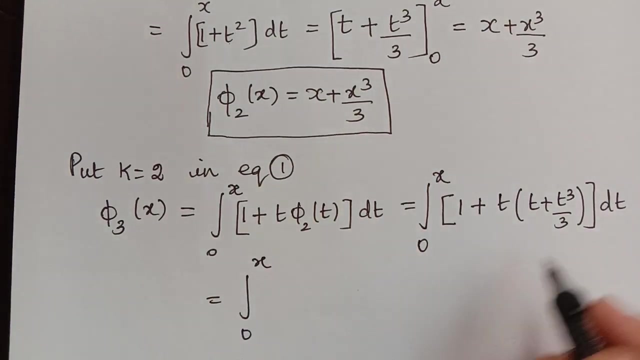 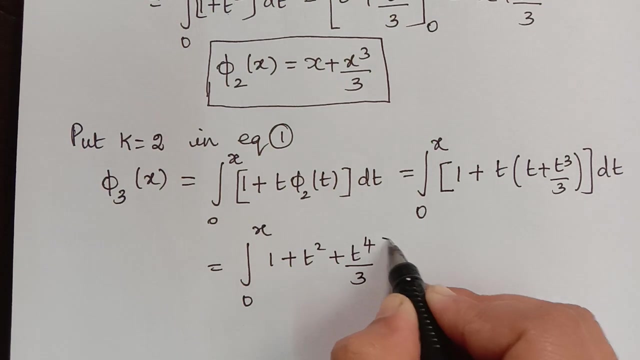 substituting that, here we get 0 to x, 1 plus t multiplied with this, that is, t multiplied with t plus t cube by 3 dt, and so that will be equal to integral 0 to x dt. And now, on multiplying this, we get 1 plus t squared plus t to the power, 4 by 3 dt. Now on,